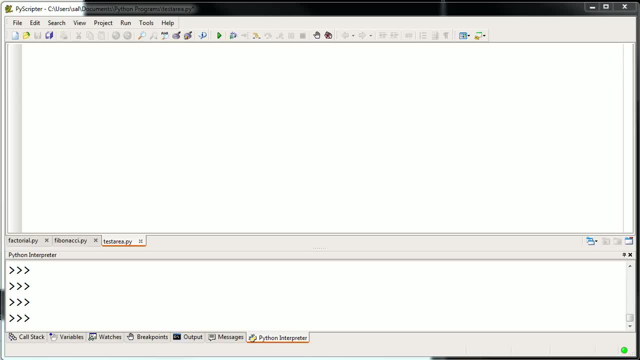 What I want to do in this video is really just expose you and introduce you to the idea of even what a computer program is. And just in case you want to follow along- and I highly recommend you do that, because the real way to learn computer science is to really fiddle with things yourself- 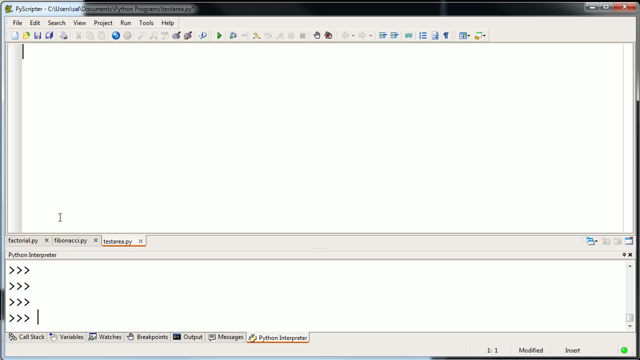 is. this is a Python environment, so I'm going to be doing a lot of the programming in Python And right here the environment is called PyScripter P-Y-S-C-R-I-P-T-E-R. It's free, it's an open source piece of software and I'm using Python. I believe I'm using Python 2.6 or 2.7.. 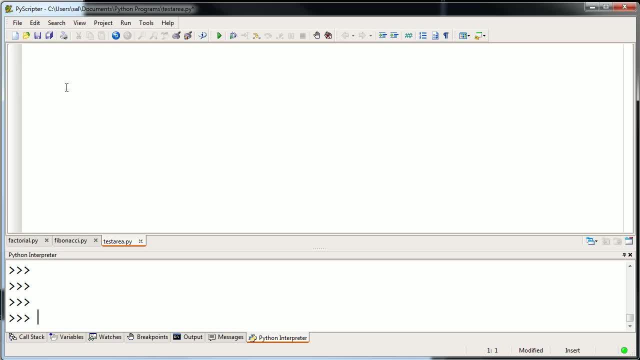 As long as you're using Python 2, your examples will be the same as mine. they'll work the same way. If you use Python 3, you're going to have to use slightly different variations every now and then to make it work properly. 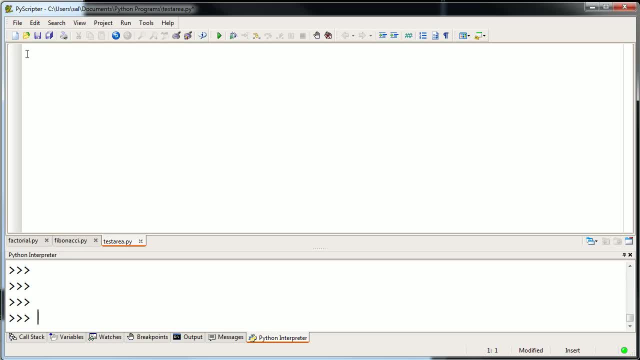 And I'll try to make notes for those when they occur. So let's just start writing ourselves a computer program. And what's cool about this is we can write our computer program right here and really we're just editing text in a file. 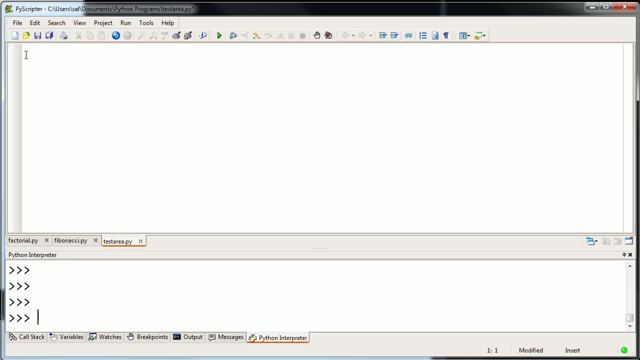 So let's just start writing ourselves a computer program, And what's cool about this is we can write our computer program right here and really we're just editing text in a file. That's all it is. it's a set of instructions and the computer is just going to start. for the most part, 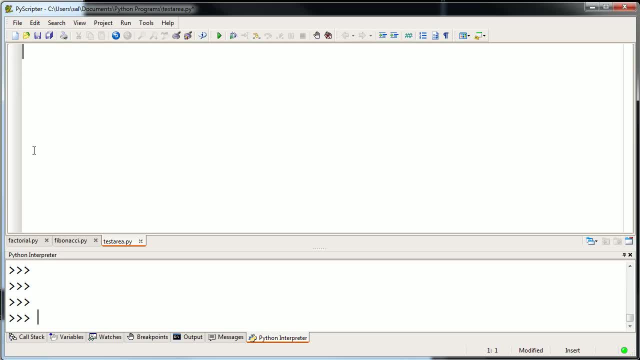 at the top of this file and just go down and read the instructions, Although you'll see later on that there's ways to tell the computer to jump around and loop around within the instructions so it can do things over and over again or skip other things. 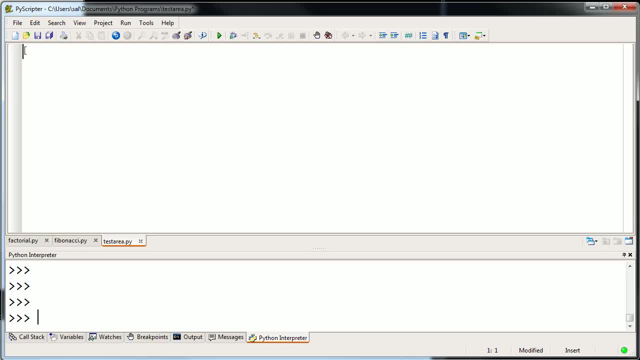 But, with that said, let's write ourselves a simple program, And while we do this, we'll expose ourselves to some of the core concepts that exist within a computer program, So one of the main. So let me just write a very, A very, very simple computer program. 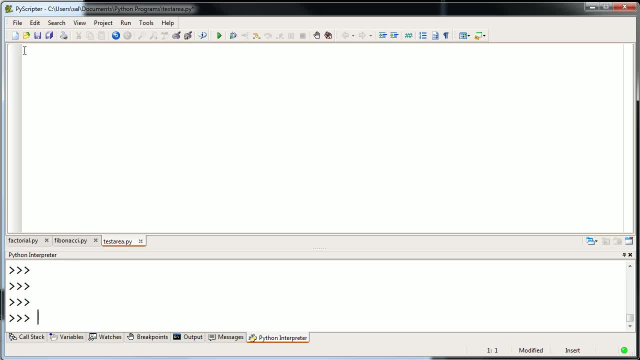 So one very simple computer program would literally just be an expression: So 3.. So let me just write: print 3 plus 7.. So it's literally just going to take 3 plus 7 and print it. It's going to pass it to the print function which comes with Python, and maybe I'll write it like this: 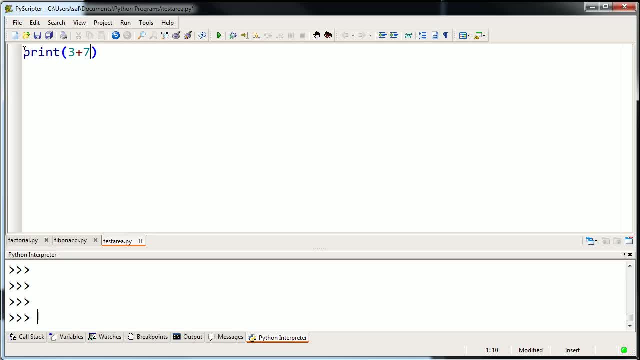 Print 3 plus 7.. And so let's save this file. So there's literally- only if you think about it- only one command. here at the top line It says print 3 plus 7.. Actually, let's add another command, just so you can see that it's going to go from the top down. 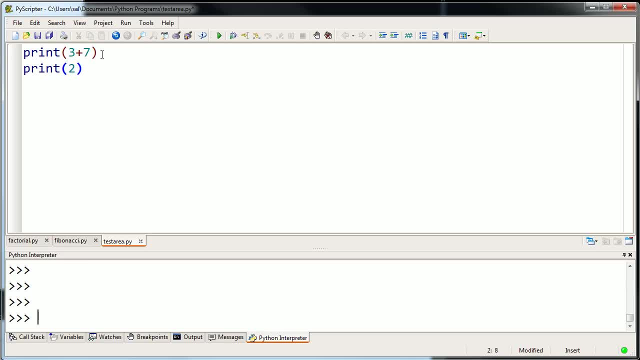 And then let me add another one: Print 2 minus 1.. And then let's do print. This is a chunk of text, And let's see what this computer program right here is going to do. So let me save it. So let me save it. 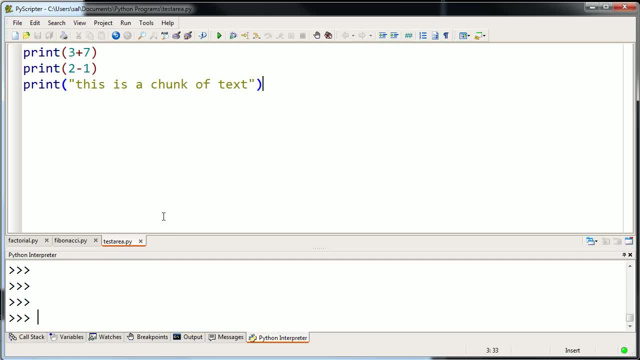 I've saved it as the file. It's called testareapy. The py signifies that it is a Python file. And now let me run the program. And what's nice about these development environments, these IDE integrated development environments, is that you can kind of type and run your programs in the same place. 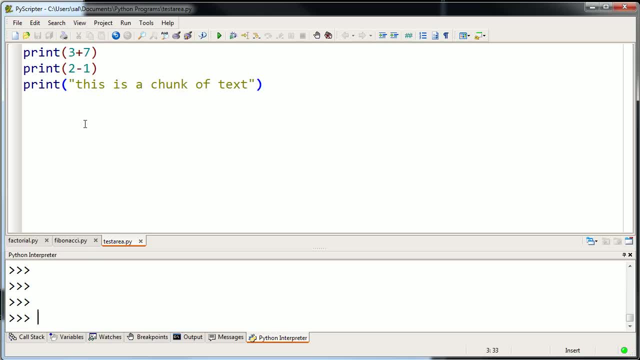 And it also color codes your text so you can see what's a function, what's not a function, the different data types- And we'll talk more about data types in the future, But let's just run this program to see what happens. 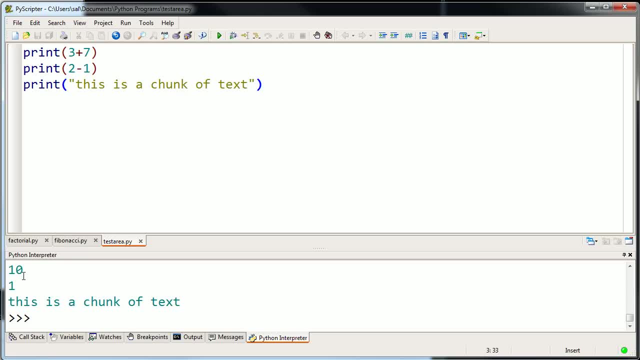 So there we go. We ran it, So it printed 10.. Then it printed 1.. Then it printed: this is a chunk of text. So it did exactly what we told it to do, And it did it in the order. 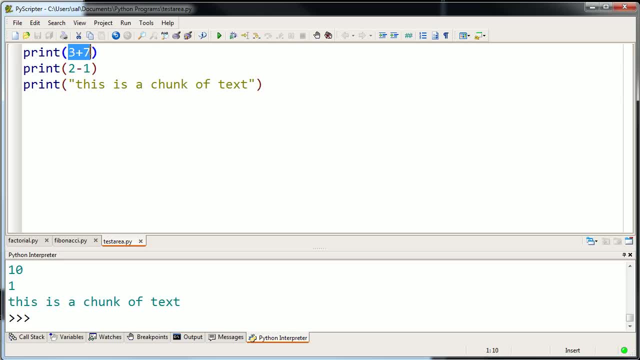 It started up here. It evaluated 3 plus 7 as equal to 10. And then it printed it. And it printed 10 here, Then it printed 2 minus 1.. Then it did that there And then it printed. this is a chunk of text. 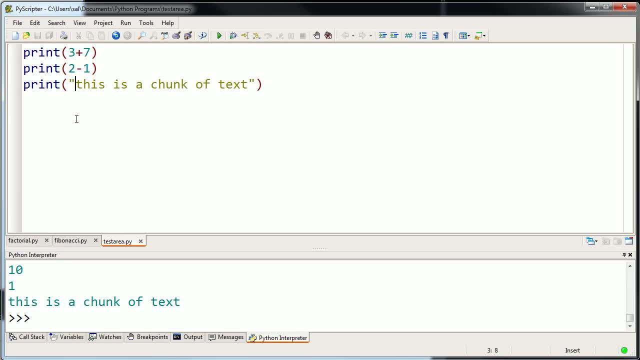 Now, one thing I want to introduce you to fairly early on is the idea of data types. So even when you saw this example, you might have had the gut feeling: But look, there's something kind of different about a 3 or a 2 or a 1.. 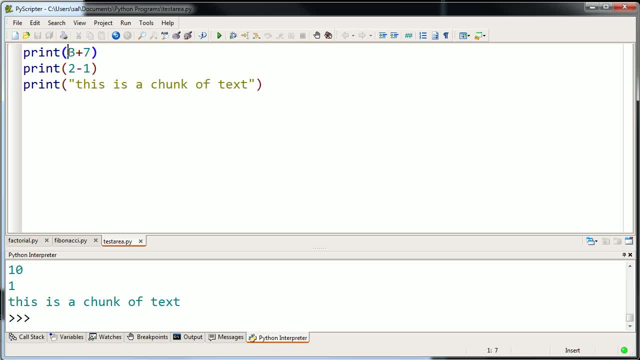 Or a 7. And this chunk of text, This is a number I can kind of just you know. I feel like I can just kind of add numbers. They're representing some type of quantity, While this over here is representing- well, it's representing a chunk of text. 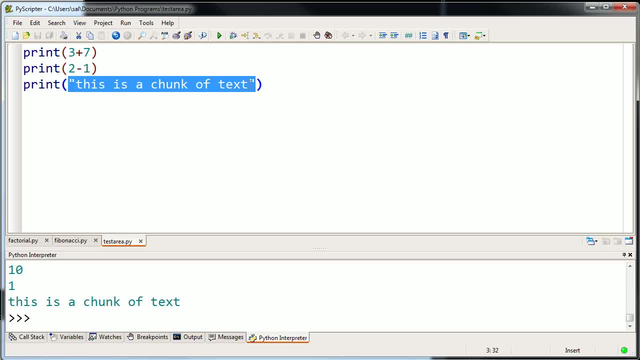 And your intuition would be right. These are different data types: The 3's and the 7's and the 1's. these are numeric literals And in this particular case they are integers. And this right over here, this is actually a string. 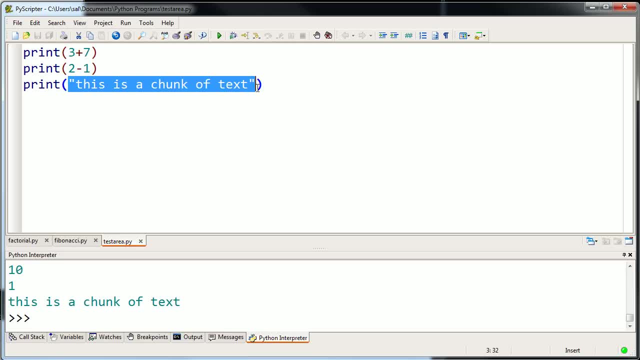 Which is a word you'll hear a lot in computer science. It's really referring to a string of characters And in Python we can actually ask it: what are the types of these things? So you can pass them to the function type. 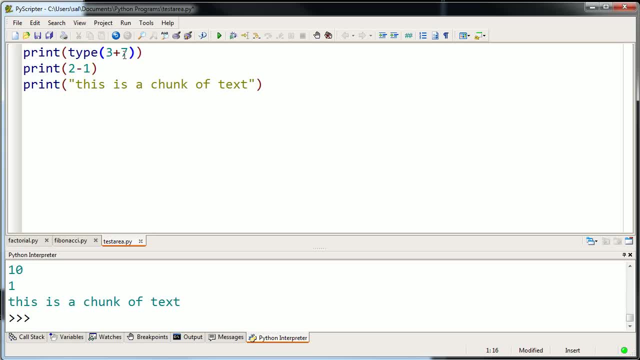 And so now it should print the type of 3 plus 7. Not just 10.. So let's try that, And I'll just print 2 minus 1 to just show you the difference, And then I'll print the type of this chunk of text. 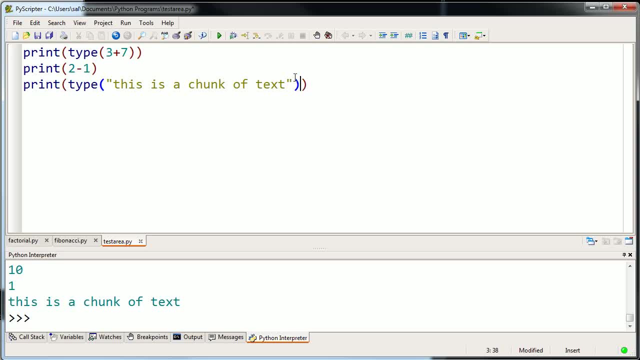 The type of this chunk of text, And so let's save it. Type control S. That's a shortcut to save this, And then I'll try to run this program. So there you go. It evaluated this statement, And to evaluate this, it starts on the inner parentheses. 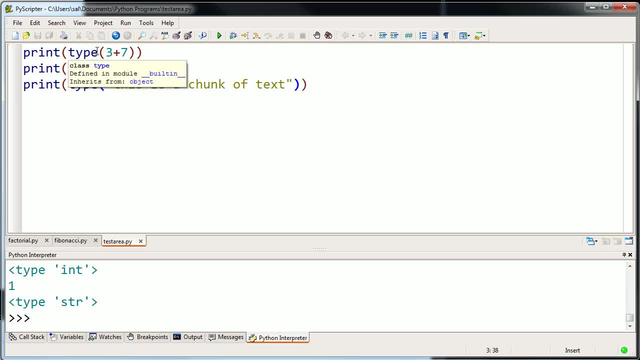 3 plus 7 is 10.. Then it tries to take the type of 10,, which is a type int, And then it prints that type int And you see it right here. It says type int. Int is short for integer. 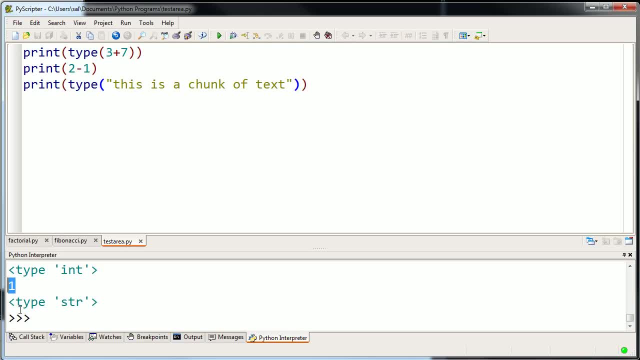 Then it says: print 2 minus 1.. It does that on this line right here, Prints 1.. And then it prints the type of this whole thing Right over here. So instead of printing it itself, it just printed its type. 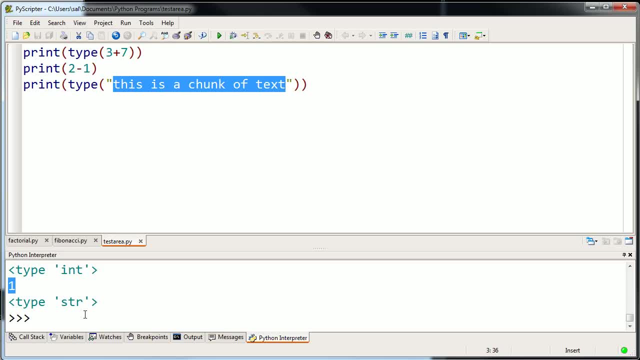 And its type is a string. Now, the next thing I want to introduce you to, as we just fiddle our way, experimenting with programs, is the idea of a variable, Because one of the things is we're going to want to kind of store these things in different places. 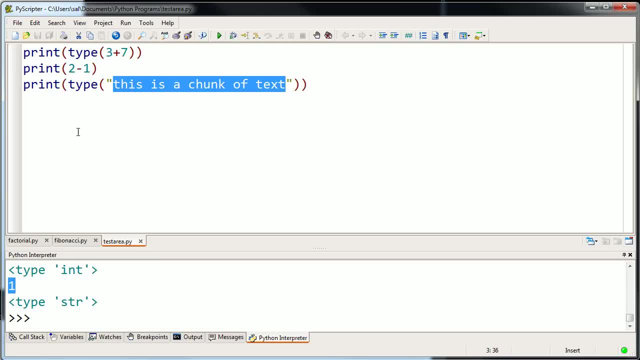 And, as we'll learn in future videos, in Python it's more of like we want to have labels on these things And the labels can change. But let's see, Or we could put them in different types of labels, So let's write a completely different program over here. 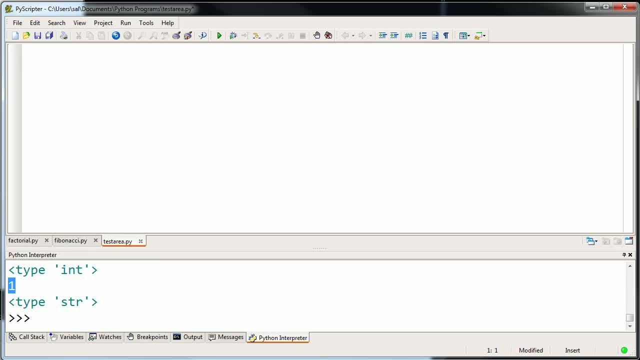 And I'll do that. I'll do it using variables, And what's cool about Python- or some people don't like it- is you could put any type of data in any type of variable. So you could say: a is equal to 3 plus 5.. 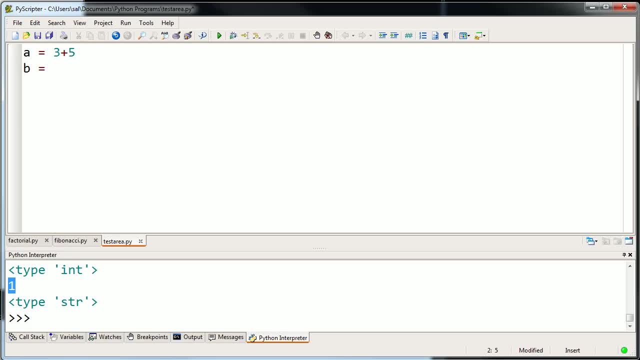 And then we can say b is equal to, let's say, a times a minus a minus 1.. And then you can say c is equal to maybe a times b, And then you could have something like: and then I'll put some space here just to make it look a little bit. 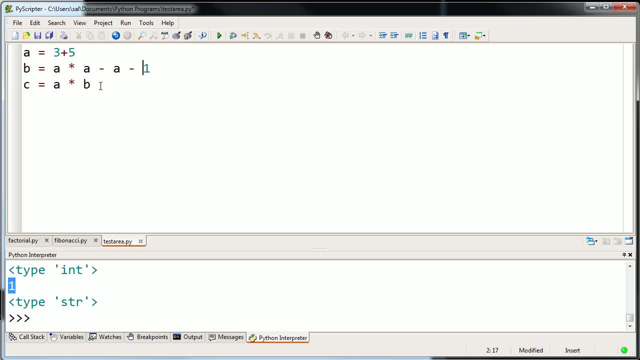 just to make it a little bit cleaner: c is equal to a times b, And then we can say: let's print c, And so, if you want, you can go ahead and try to figure out what c is going to look like. 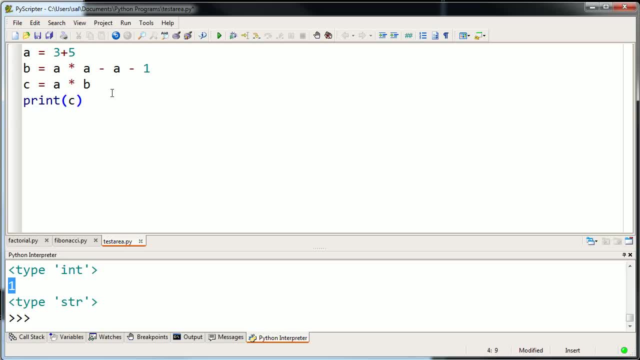 Or we could just run this program. So let's run the program first, And then we can go back to see that it actually did the right thing. So I'm just going to save this program And now I'm going to run it. 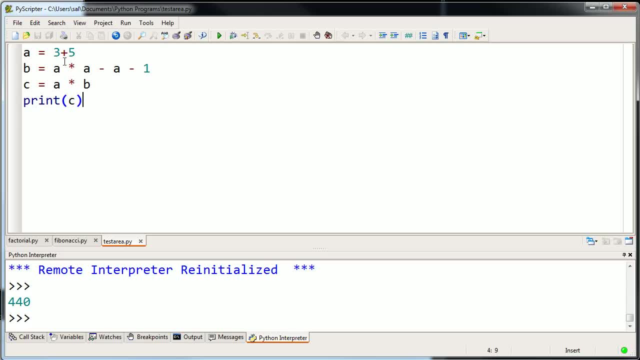 Well, I got 440 for c, So let's see if that makes sense. So 3 plus 5 is 8. And so the label a will refer to 8. So any place in the program until we redefine a. 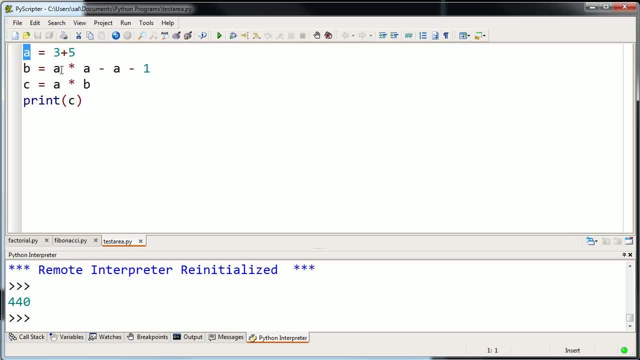 any time you use a, it's going to say, well, a is an 8.. a is referring to 8.. So when you go down over here and we're defining b, it'll say OK, a times a. 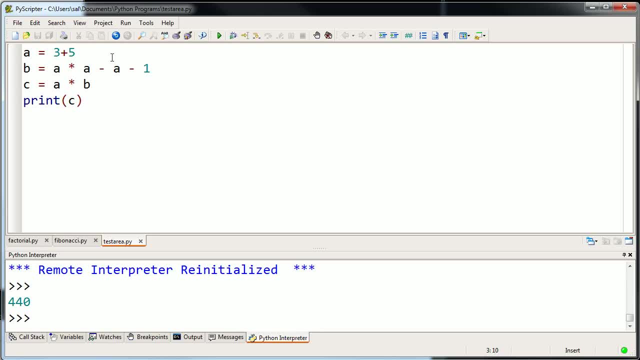 And it uses order of operations. So in order of operations, you do your multiplication first, And so a times, especially when you're comparing it against subtraction, So a times a, that's going to be 64. And then we have 64 minus a. 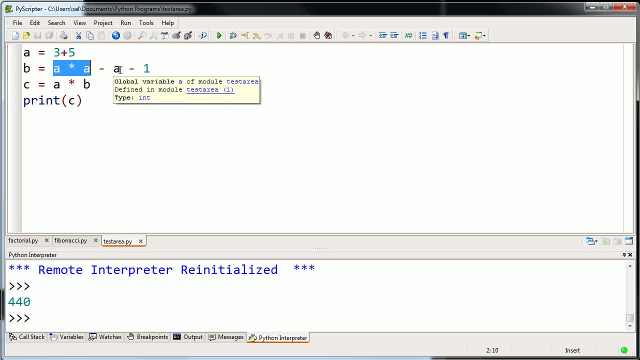 So 64 minus 8 is 56.. Minus 1 is 55. So b is 55. And then c is going to be a, which is 8, times 55. And 8 times 55 is indeed 440.. 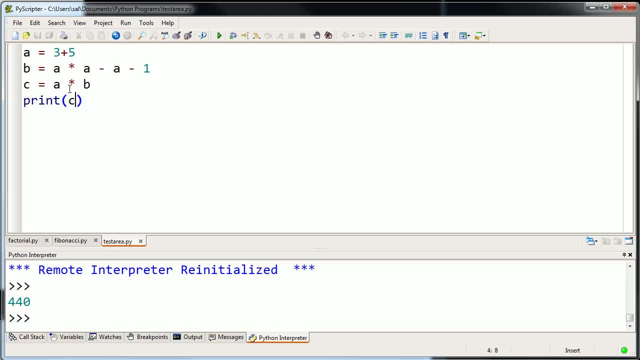 So it all worked out And so maybe you define these things and you want to see what happens when you get different a's And you can try that out. You can just change what happens here for the different a's, So maybe we'll have a is equal to negative 6.. 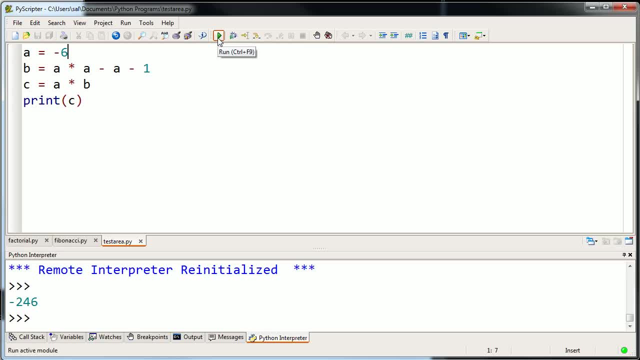 Now let's run our program and see what happens. We get negative 246. And you can verify it for yourself. You go line by line and have these variables refer to what they're defined to be referring to and see if you get this response right over here. 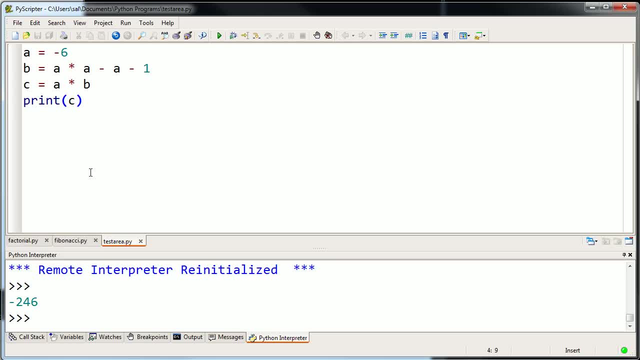 Now, if programs were just a bunch of commands that you just always go straight through, you wouldn't be able to do really interesting things. And so to do really interesting things, you're going to start seeing things like conditionals and loops, And a conditional and a loop is something like. 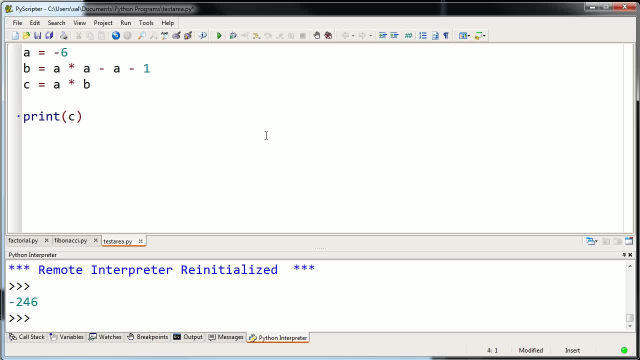 let's do it like this. So, if so, I'll just leave that stuff over there And we'll say: if a is less than 0, maybe we will print c, And if or else print, let's print. otherwise we'll print c minus. 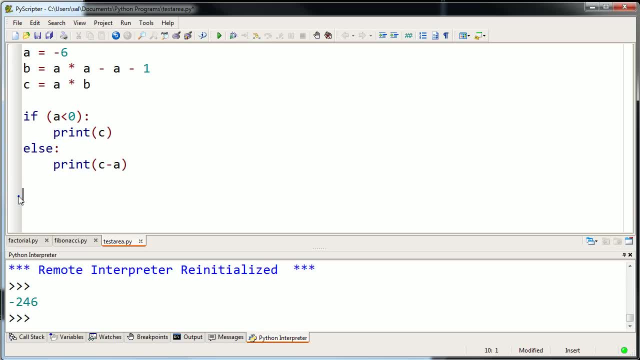 otherwise we will print c minus a. So this is interesting And you might already have a gut for what's going to happen here. but let's save it, And it's amazing how much you can get done with just these conditionals. So this is saying: if a is less than 0, do this. 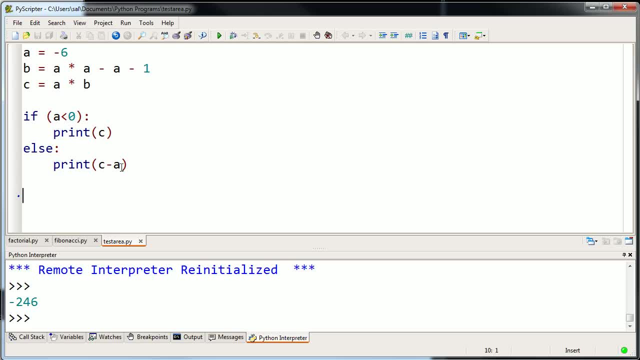 Otherwise, if a is not less than 0, do this over here. So notice, we're not just going to go straight down Depending on whether a is less than 0 or not. it's going to either execute this line or it's going to execute this line. 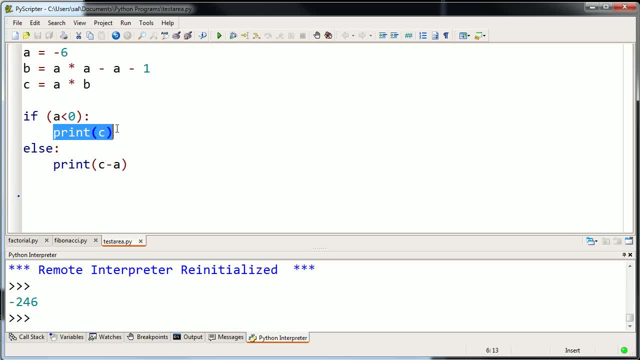 And the way that Python knew to only execute this line if a is less than 0 is it's indented here And the indent it's part of this clause, And the way it knows that there are new clauses forming right here is this colon right over here. 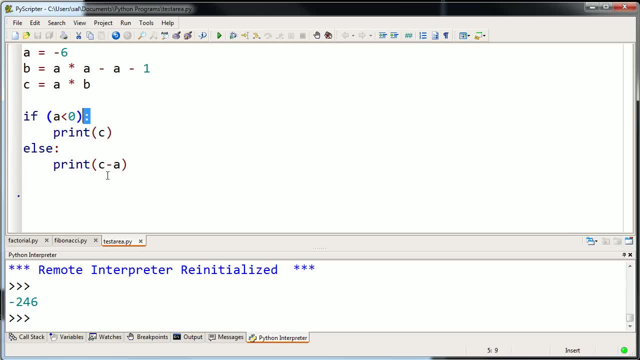 And then the way to know what to execute. if none of this happens, or if a is not less than 0, it's within this else clause, And if you want to do something else after this, regardless of whether a is less than 0 or not, 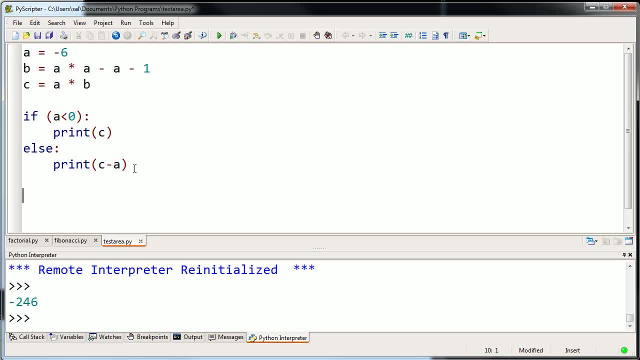 you just take it out of the clause by getting rid of the indentation. So now we can just print and we are done with the program. Actually, let's add some other stuff in this clause. So let's print here: a is less than 0.. 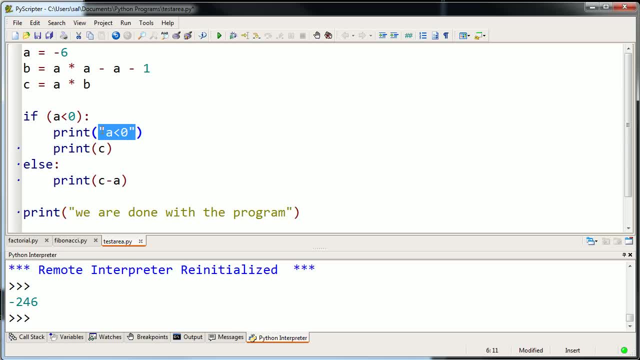 So notice, this is not going to be evaluated. We have this inside of a string, So it's just going to print that thing And then over here we'll say: print a is not less than 0.. So this is an interesting program. 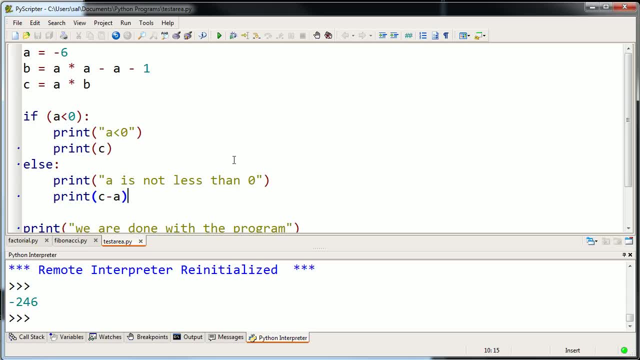 Let's just run it now. All right, let's hope it runs. All right. so I saved it and now let's run the program And it says it printed a is less than 0.. So if we could scroll up a little bit,